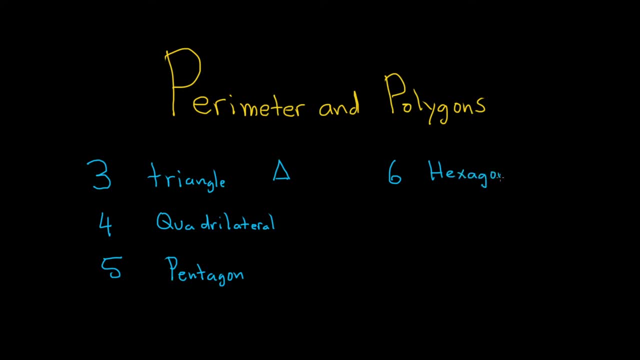 A little more obscure perhaps If it has seven sides. this one's even more obscure. It's called a heptagon- Really fancy names, And we'll stop at eight. Eight is called the octagon. So those are the common polygons. So the perimeter is the sum of the lengths of the sides of a polygon. 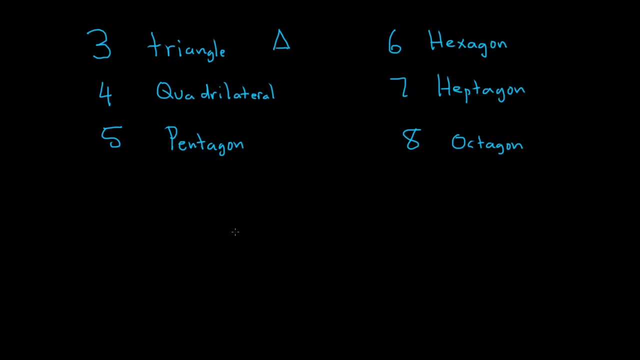 Let's do some simplification. Let's do some simple examples. Let's say we have a triangle Looks like this, Okay, and let's say that this is 12 inches, 17 inches and 19 inches. So if you had to find the perimeter, all you would do is you would add everything up. 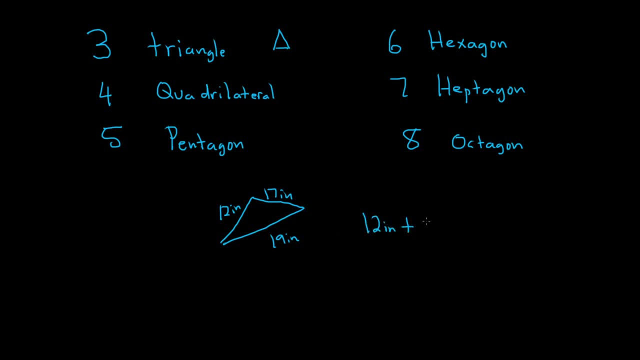 So you would do 12 inches plus 17 inches plus 19 inches. You're probably wondering: do you have to find the perimeter? Do you have to write the inches every time? The answer is not really, but you just have to make sure that you include the inches in your final answer. 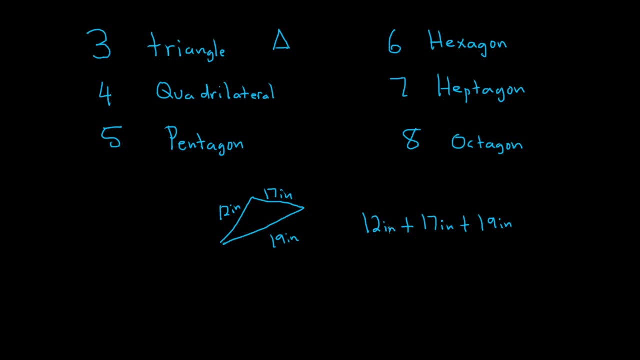 Okay. so most of the time people really like it when you write the inches. So if you're doing this, like for a class or something, just check, You know, you might, you might, they might want you to write it every time. 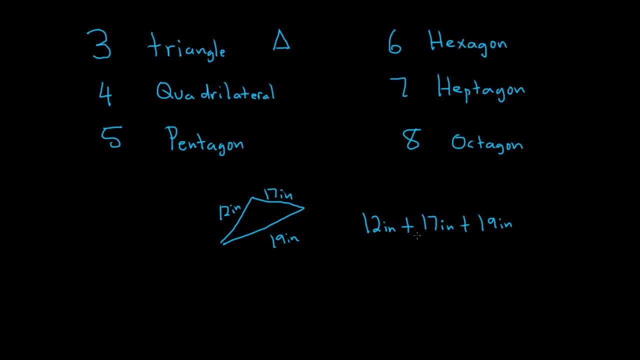 So if you add all these up, I'm going to cheat and use a calculator. So 12 plus 17 plus 19.. I got 48.. So this is 48 inches. So that would be The perimeter And again, it's really important to include the inches. 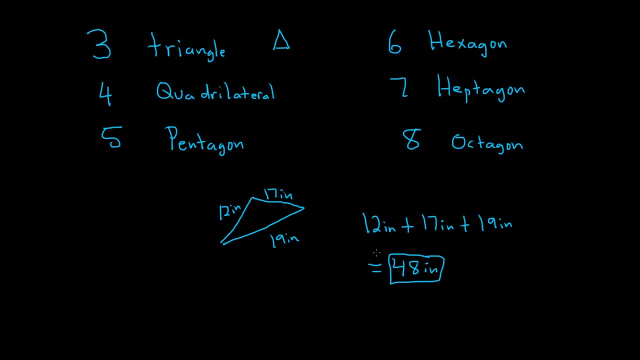 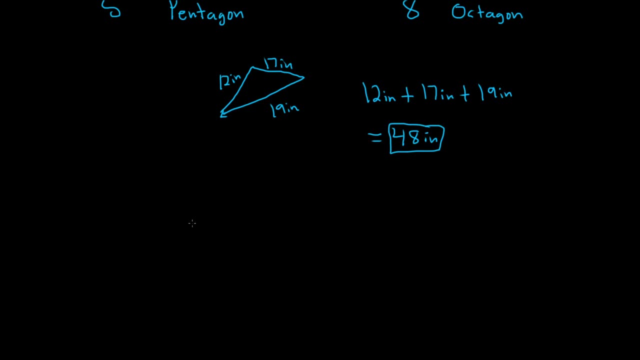 The inches is part of the answer. okay, It's part of the answer. So this was, by the way, a triangle, right, Because we have three sides. Let's do another example. Say, we have something like this: So here we go. 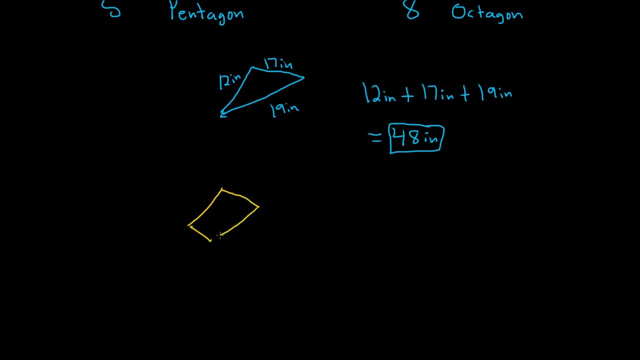 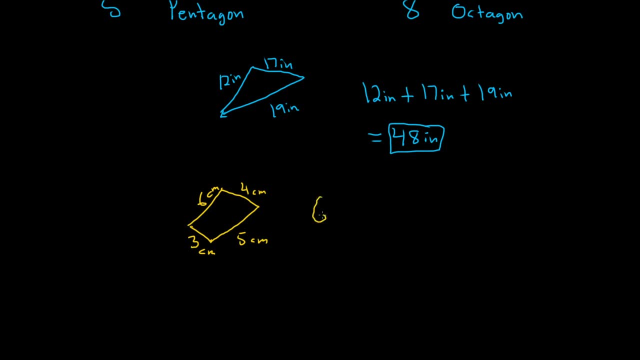 So to find the perimeter we would just add up the lengths of all the sides, So you do 6 centimeters, And it doesn't matter which one you write first. okay, Plus 4 centimeters. plus 3 centimeters. plus 5 centimeters.